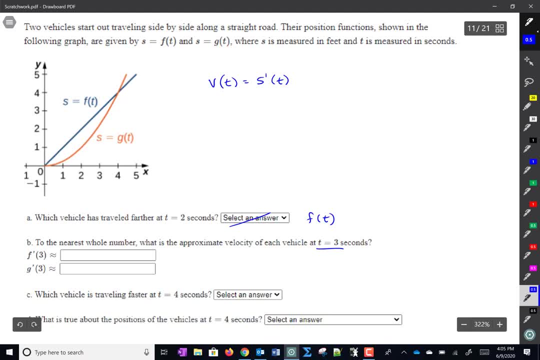 And the point in question here is where t is equal to three. So where t is equal to three is right here, And this point is on the function f and this point is on the function g, Now the tangent line to a. 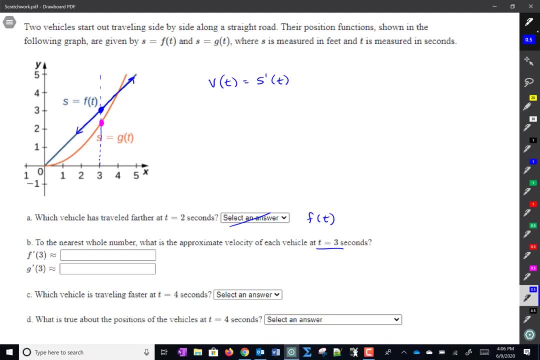 Maybe I should have used a different color than blue. But the tangent line to a line is just equal to the line, is just equal to the slope. So the slope of the tangent is just the slope of the line, And approximating the slope of this line, 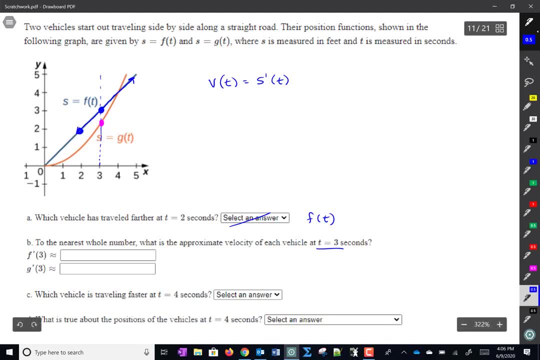 if I go from this point, which is on the line, to this point, it looks like if I go up one and then over one, then that gives me an approximate slope of one over one, which is one Now for the other function. 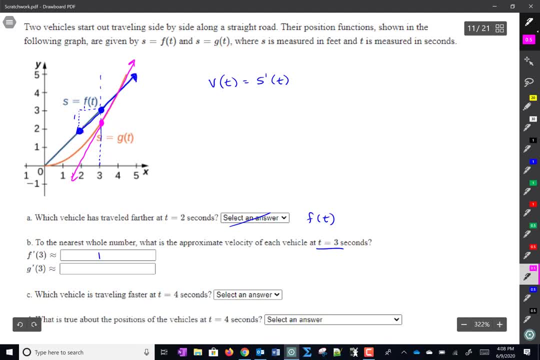 this tangent line looks a bit steeper And we need to get an approximation as to just how steep that is. This is close to the point three, two, the way I've drawn it. We'll just approximate that. And then this point right here: 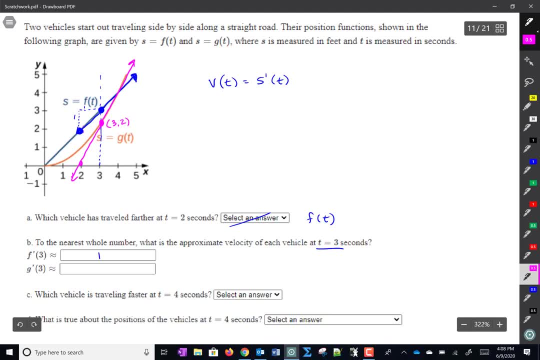 looks like it's at two zero. Okay, So if we go from this point to the other, it looks like we need to go up two and then over one, And then two over one gives us a slope of two, So that gives me an approximation there. 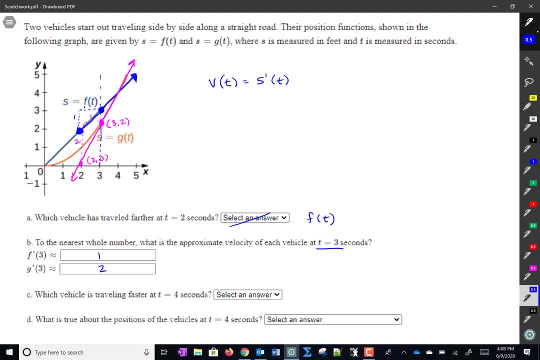 Which vehicle is traveling faster? at t equals four. Well, at t equals four. the slope of the tangent line is of function g is larger than the slope of the tangent of f. So g of t is traveling faster there. And what's true about the positions of the vehicles? 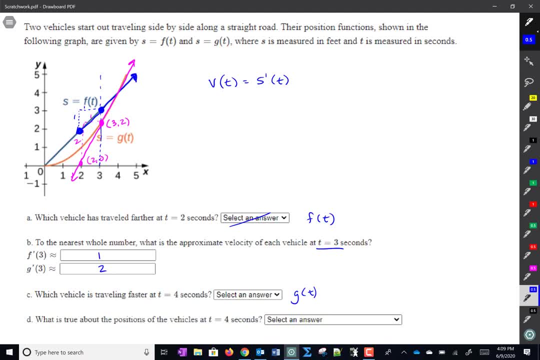 at t equals four seconds, The two vehicles are at the same position, So their y value agrees. And if they're at the same position, that means that they're at the same place. So whichever answer is closest to that, So the vehicles are in the same place. So we'll write here: the point of the tangent is larger than the slope of t, three times greater than t. So therefore, g or t is that the point at which the car is at is less than the slope of t, And so g of t gives us a slope of t. We'll write: g of t is the deviation, So g of t is the deviation. And g of t is another constant to the one which is greater than t, And so g of t is the deviation. 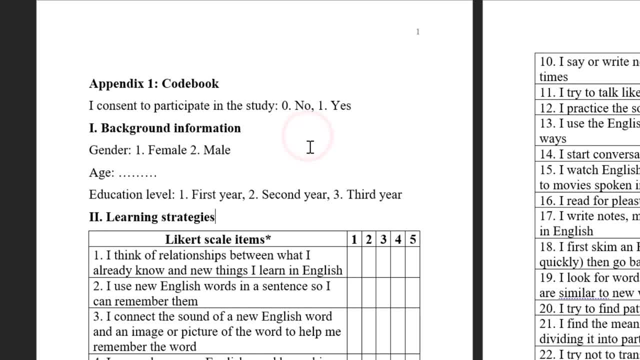 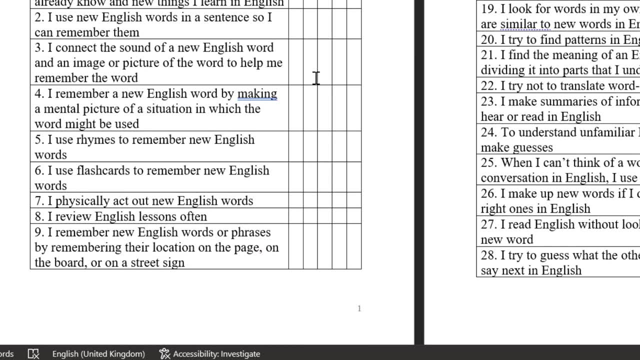 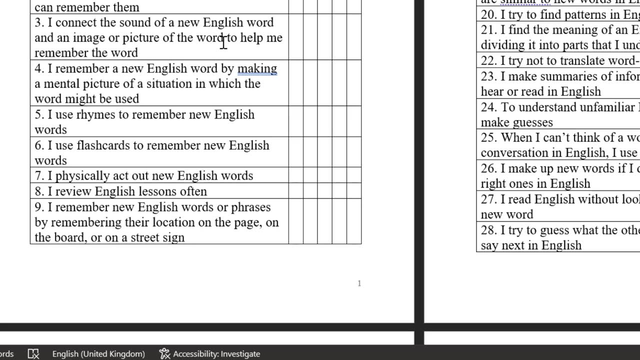 Hello everyone, I hope you're doing great. In this tutorial I'm going to share with you how to analyze record scale using descriptive and inferential statistics and interpret the results. So we have this questionnaire that is on learning strategies- inventory. that is adapted from Oxford. 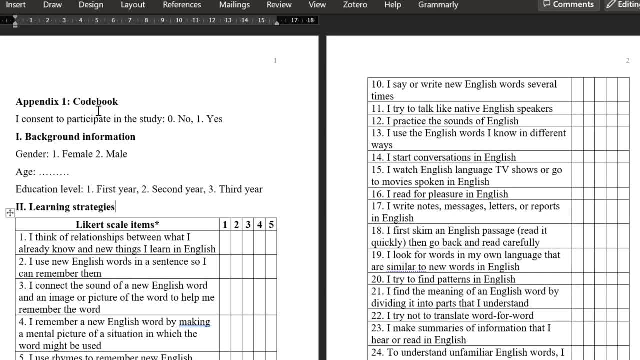 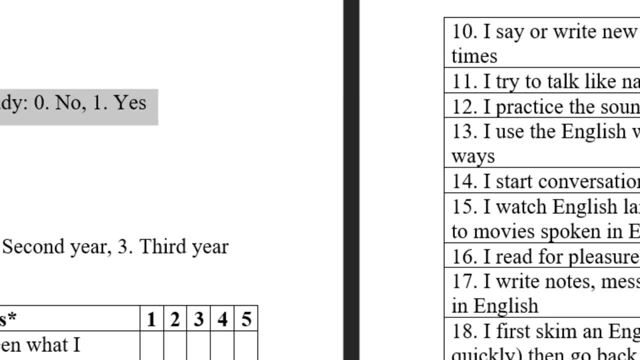 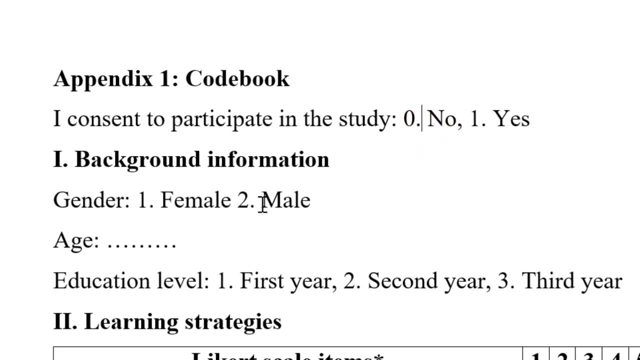 and we need to analyze it. So, before analyzing this survey, we need to have a code book like this. So I need to code the items as you can see: one or zero for no and one for yes. for gender, we have one for female, two for male. age is a continuous variable. sometimes it has categories. 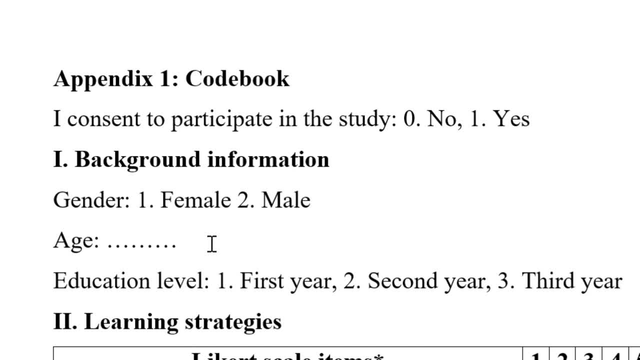 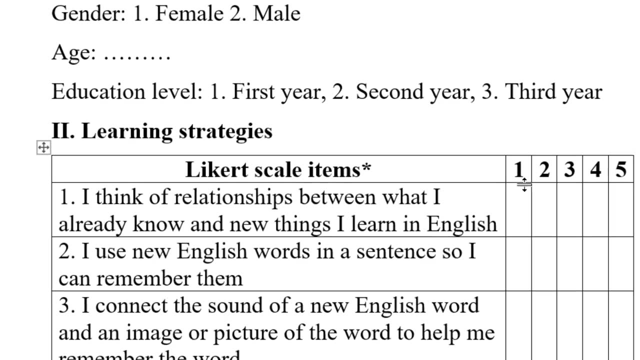 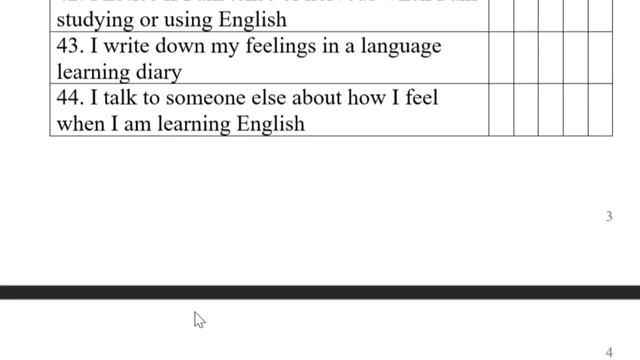 so we can code them respectively and we always assign the lower values to the lower categories, because a spaces or excel just understands numbers, not a statement like this. So anyways, once we do the coding, we code also the lacquer scale items from 1 to 5, and we do this from strongly disagree: coded as 1, that is the lower value, and strongly agree: coded as 5,, that is the highest value. 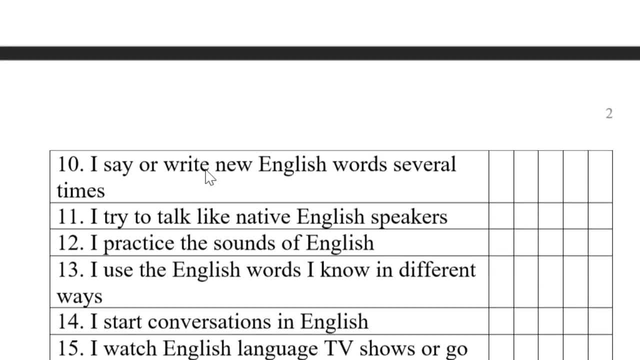 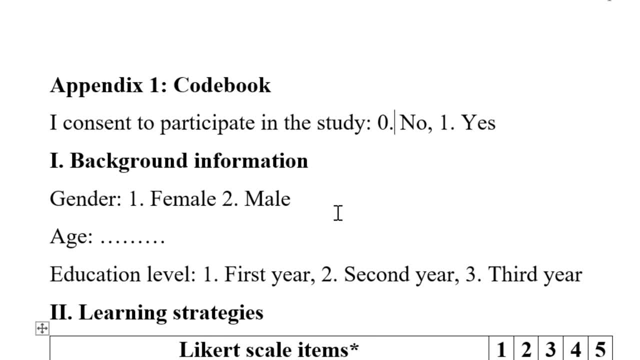 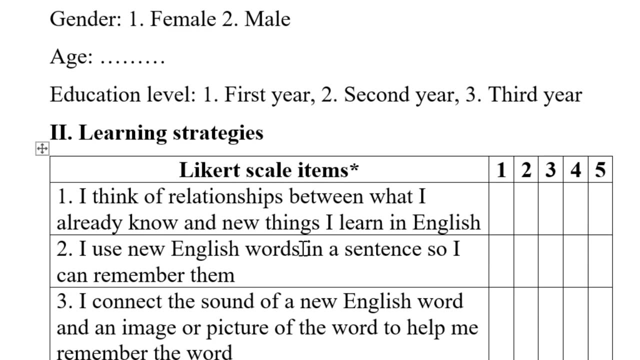 Then once we code the survey, we can code it also on Google Forms or Excel or Microsoft Forms or any platform that we use to get the data. I'm going to attach the video on how to code the questionnaire on Google Forms or X in general or CSV file very quickly. 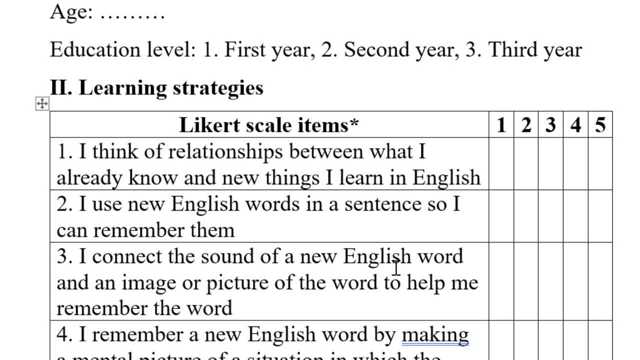 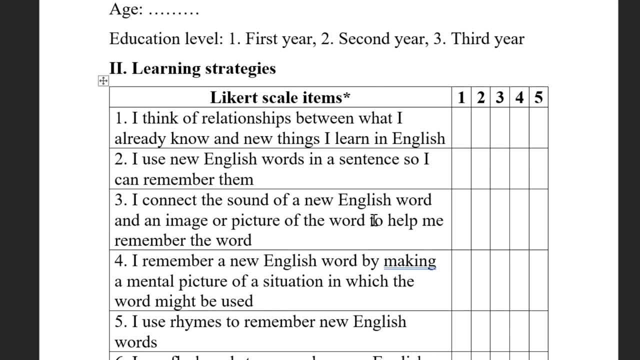 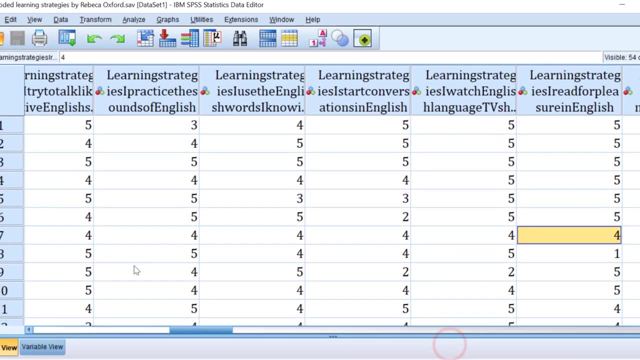 So, once we code the questionnaire, the next step is code the data, of course, and then we can either analyze it Using Excel- in that case we are just going to use certain formulas- or we can use it. we can just analyze it using a spaces, and that's what I'm going to show you.